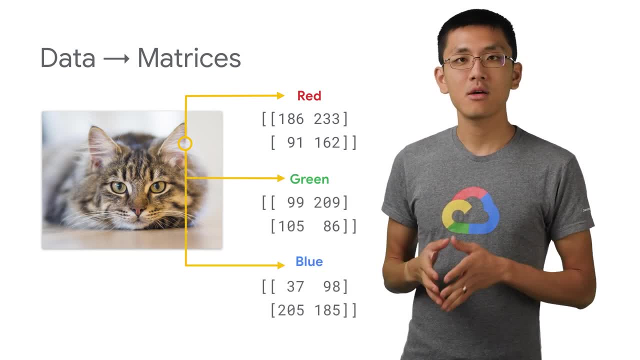 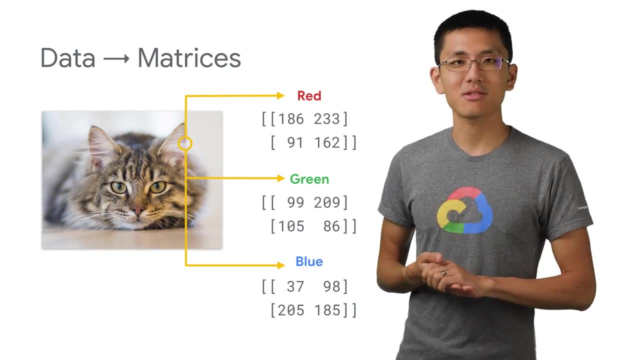 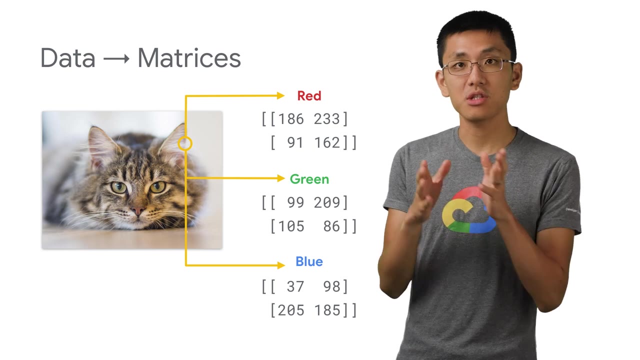 we aim to turn our data into matrices or tensors. This is very natural for images, since that's already their inherent representation. Structure data often meets a similar fate with numbers in a spreadsheet mapping very directly to input matrix values, But with natural language. 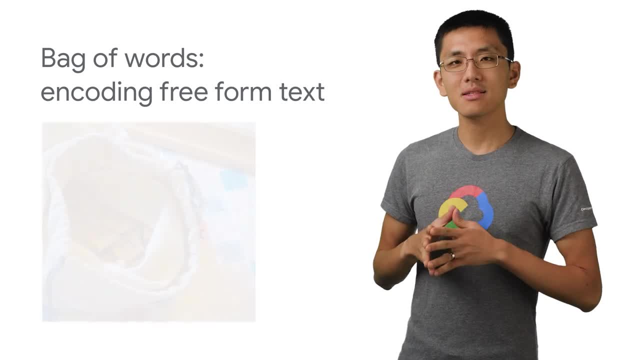 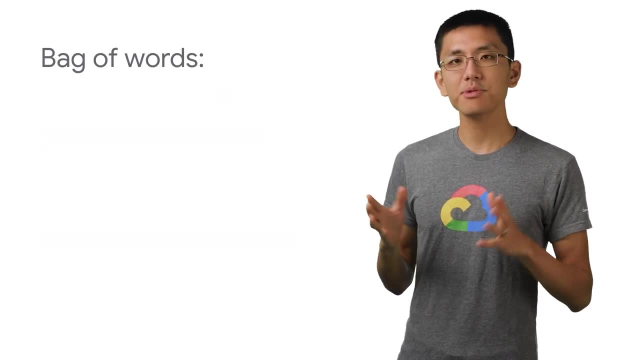 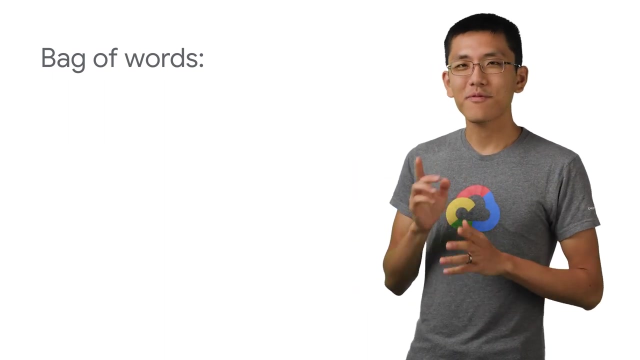 can stick them into those matrices. There are many ways that we can do this, And today we'll focus on an approach called bag of words. Let's pretend for a moment that we're learning English for the first time ever And, for some reason, the first words 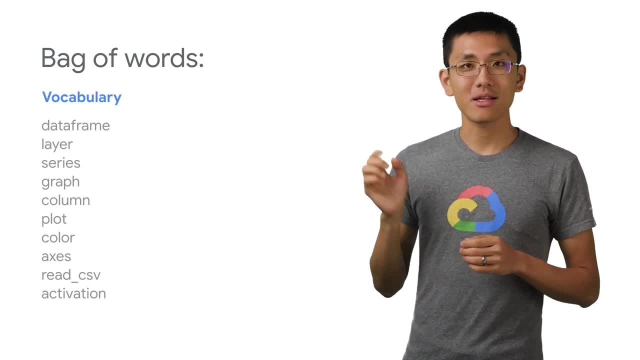 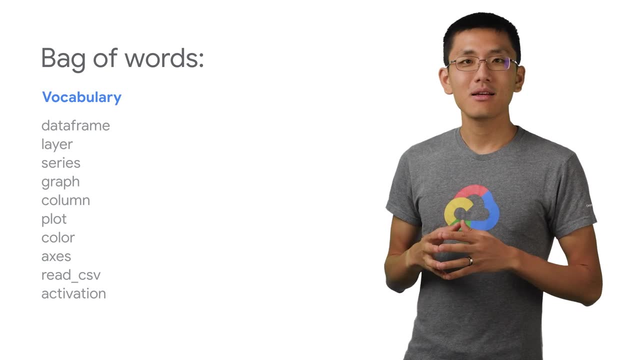 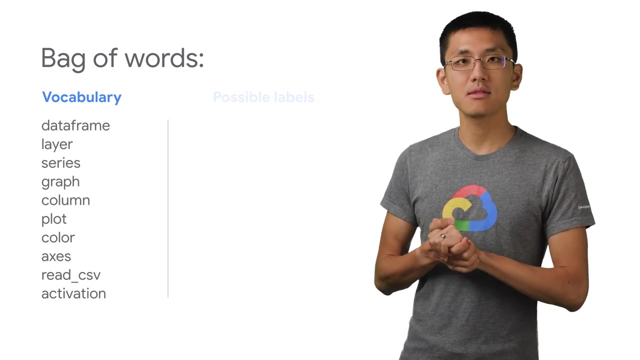 we have chosen to learn in our entire vocabulary. well, are these 10 shown here, words like data frame and graph, plot, color and activation, And so we want to be able to identify, given some arbitrary text, whether that topic is. 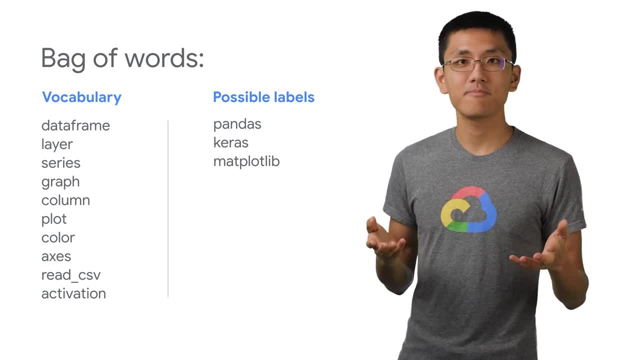 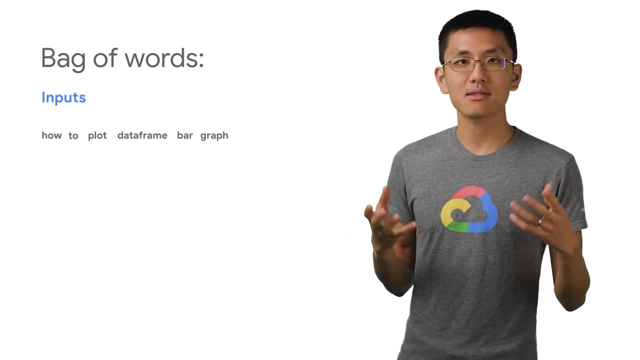 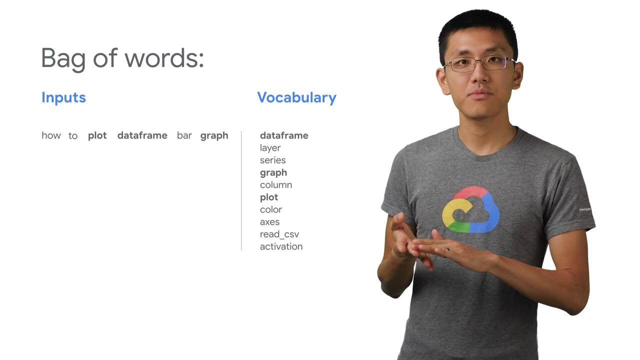 about pandas, charis or matplotlib. So how might we do that? Well, perhaps if we looked at a sentence like how to plot data frame bar graph, we would recognize just the words plot, data frame and graph. The rest of the sentence well it. 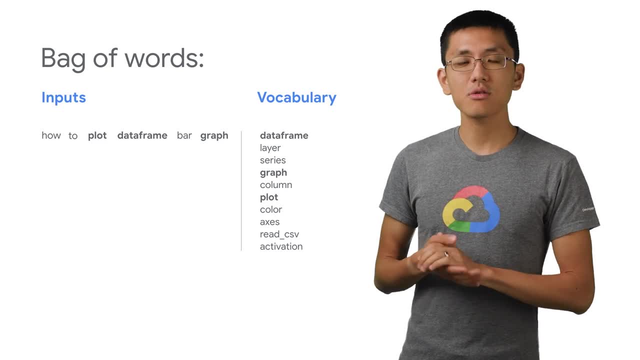 would look like a foreign language, just gibberish. Knowing only those three words in the sentence, though, we might still be able to get some sense of what it's about, And the way you might capture this information in an array or matrix would be to first make. 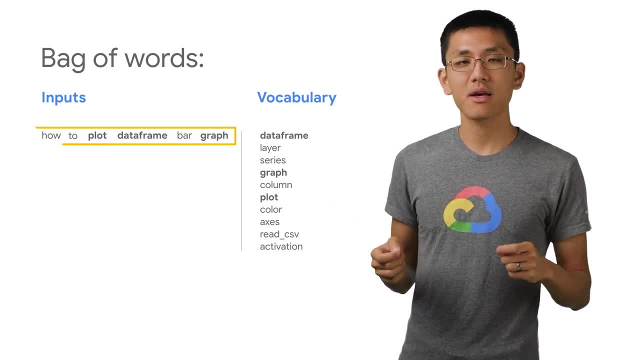 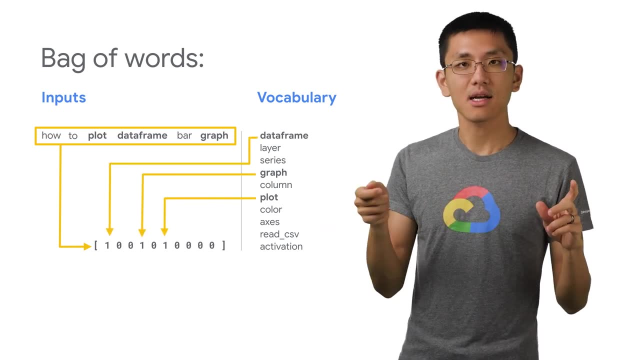 an array that represents your entire vocabulary. So in this case we have an array of just length 10.. We'd set all those values to 0 and turn on the array indices that correspond to the words in the sentence by setting them to 1.. 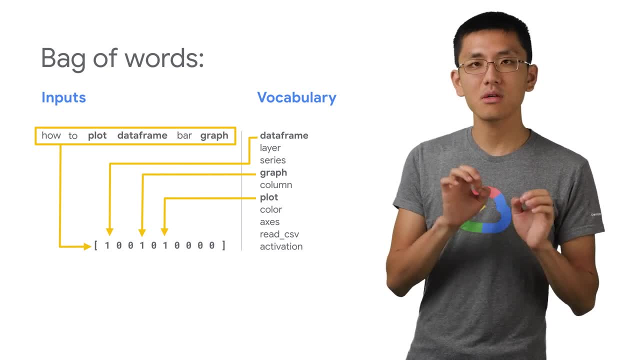 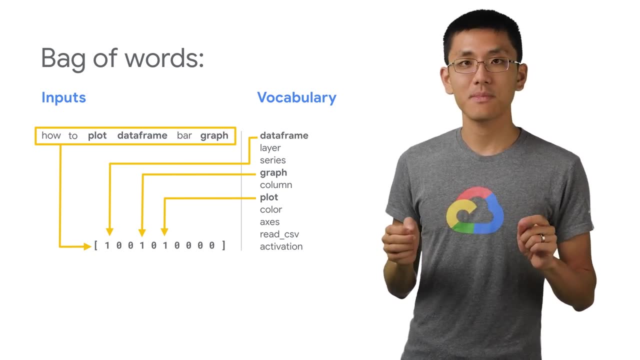 Notice that this has a little bit of a difference. It has nothing to do with the order the words appear in the input sentence, but everything to do with the order of the words in our vocabulary list. So now we've encoded or translated the English sentence. 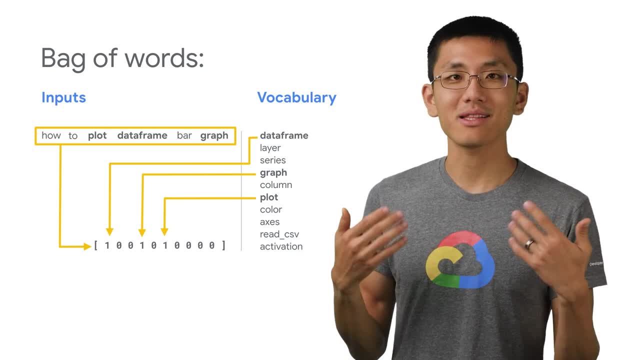 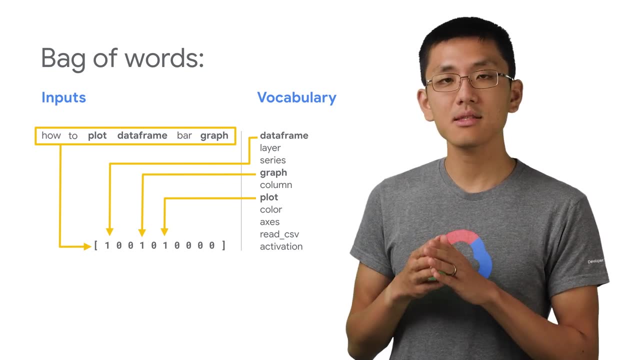 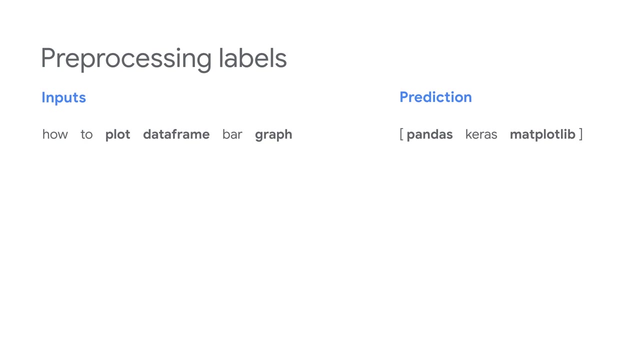 into an array of numbers based on our well, somewhat limited understanding of English. The words we don't recognize, we'll just ignore. Notice that this has the effect of scrambling up the order of the words like, say, a bag of words. 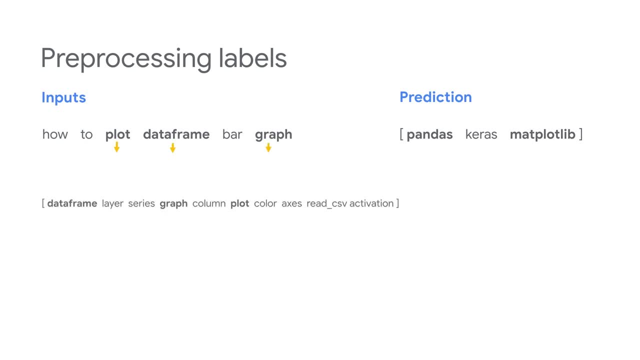 Of course, we should do the same for our labels. This is much simpler, since there are only three of them In our case, we have some sentences that have more than one label attached to them at the same time, however, since a sentence can talk, 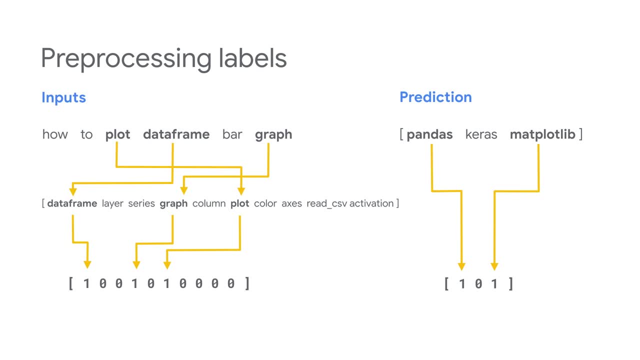 about multiple topics at once. So in that case, we want to set all the relevant indices to 1,, leaving the rest at 0,, just like we did for the words from our training data. Now we've turned the input, We've turned the output, as well as. 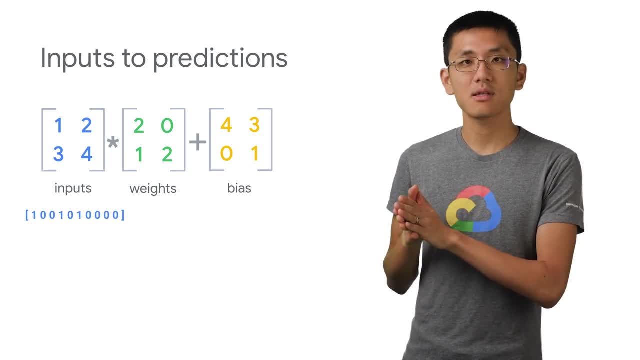 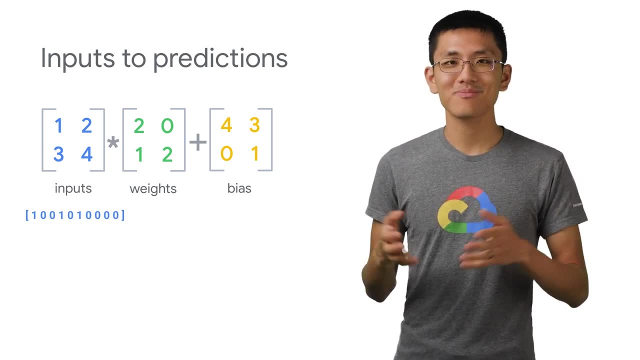 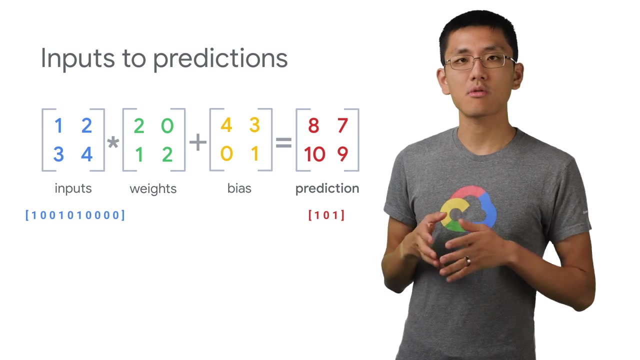 the outputs, which both used to be words, into arrays of numbers, And we can let machine learning do what it does best: map one set of numbers to another set of numbers. All the heavy lifting is done in the preprocessing, as we transformed or encoded that text. 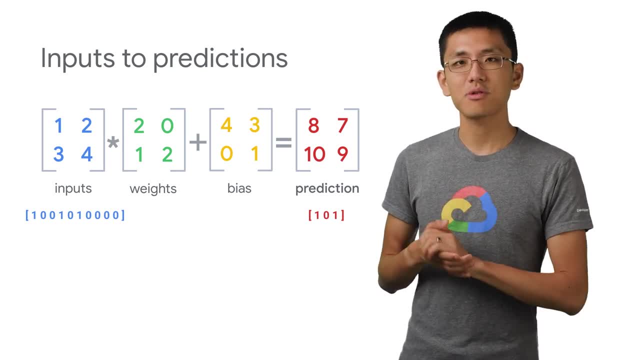 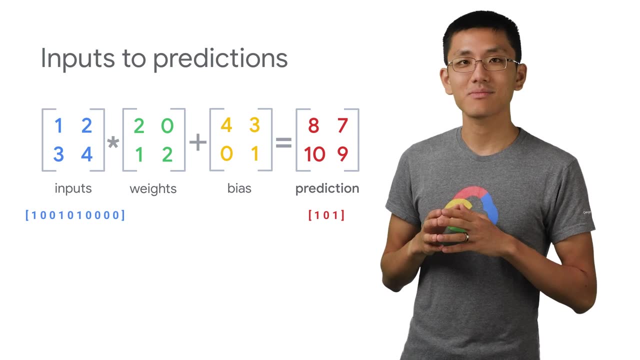 into numerical representations. Bag of words is a pretty simple approach for doing this task, though it's worth pointing out that it might surprise you how well it works in some situations. OK, So how might we build a bag of words model with code? 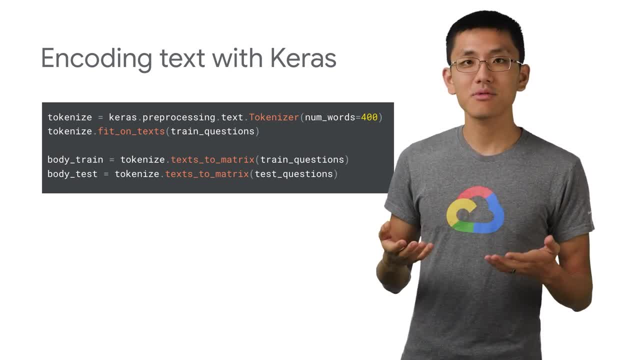 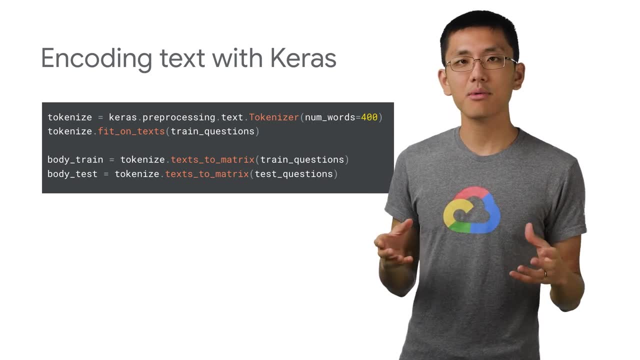 Keras has a convenient preprocessing library that we can use to handle much of this. for us, Using the tokenizer class, we can select the size of the vocabulary we'd like to utilize. In our example, we just had 10 words, which is quite small. 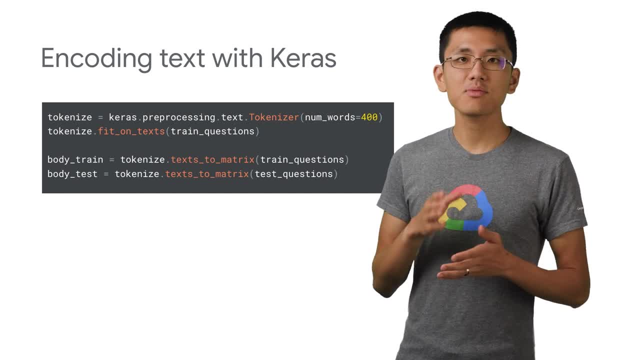 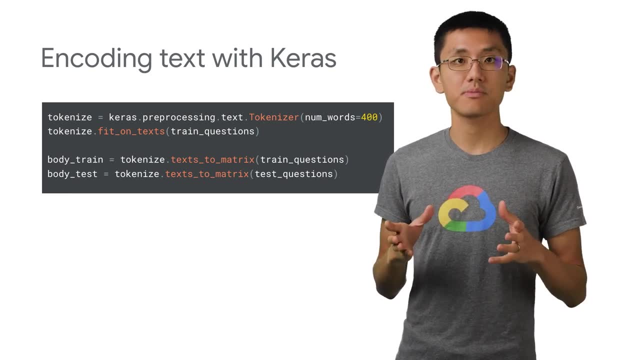 But in our code let's choose something bigger, like 400.. This will then be fit on the entire body of the text from your training data, selecting out the most common 400 words, With the tokenization process, complete building the model becomes quite straightforward and similar. 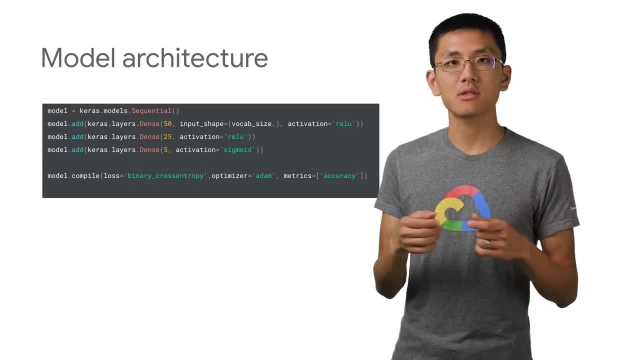 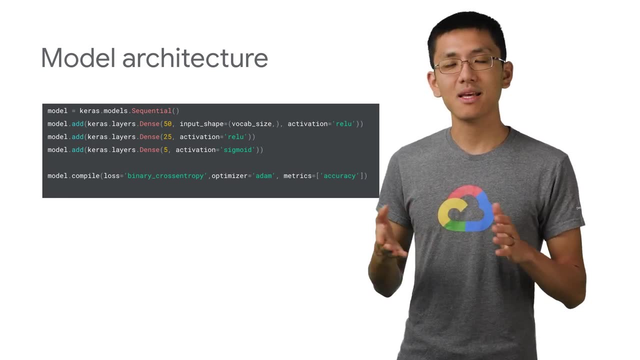 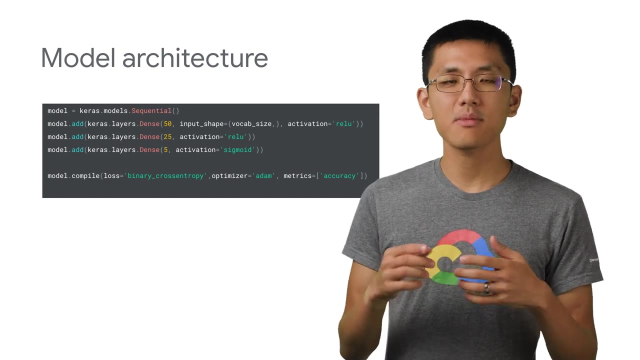 to working with other structured data, Since each row is now just an input of ones and zeros. using something as simple as a standard fully connected deep neural network can be quite effective If you're planning on having multiple label classification, where more than one label might be. 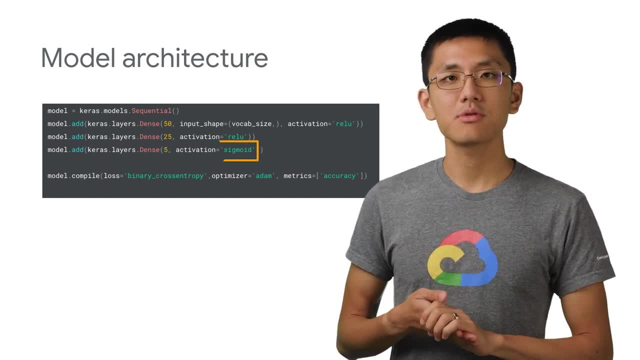 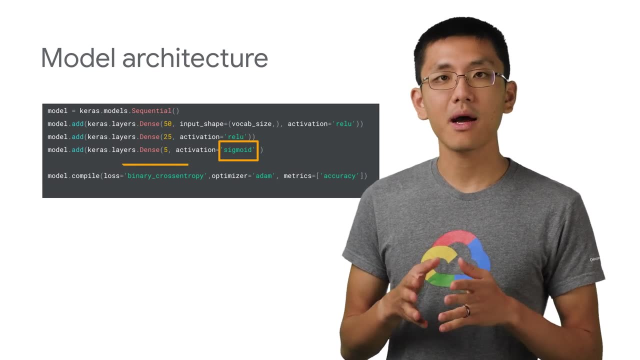 true for a single input, as we do here. be sure that we've done that, Be sure that we choose a sigmoid activation instead of the more common softmax activation function and pair it with binary cross entropy loss. So there you have it, the bag of words model in a nutshell.